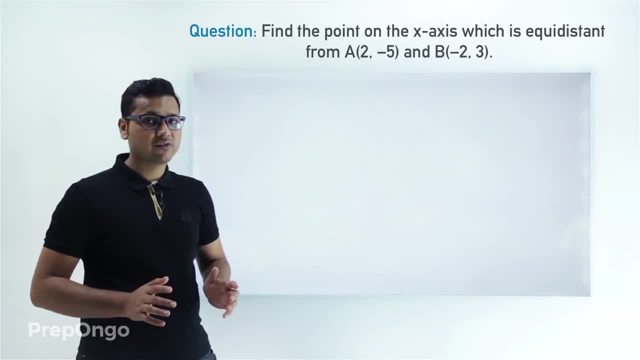 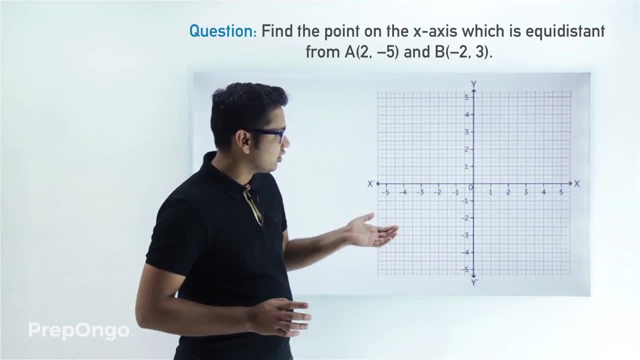 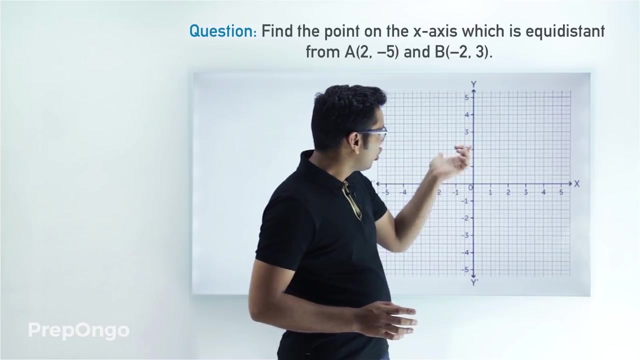 from A and B. So before proceeding, let us first plot these points A and B onto the graph. So here is a graph and on this we'll plot the points. So if you look at A, it is So we will say that 2 will signify that it is at a distance of two points from the origin. 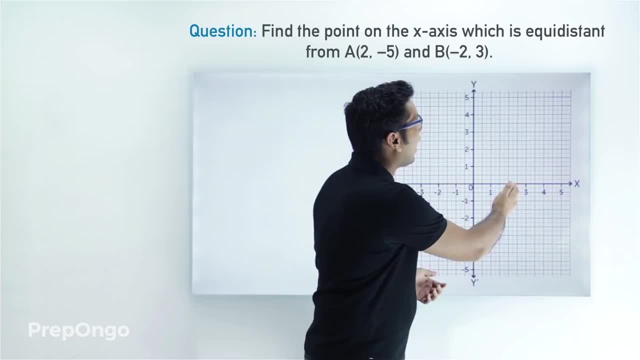 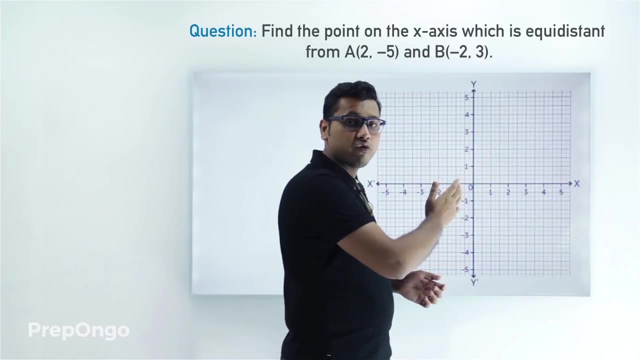 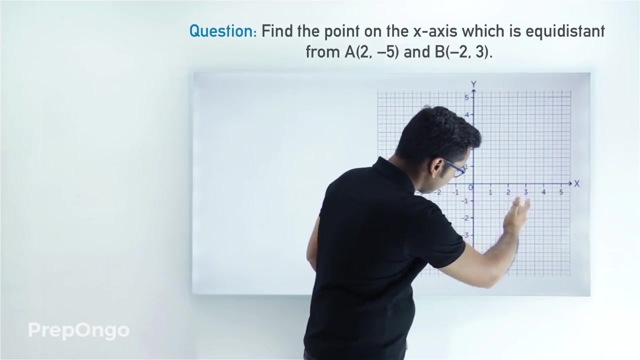 on the X-axis, so it will be here, and if we see the, so it will be at a distance of five from the origin in the y-axis 2.. so we'll move down 5 points. so this is minus 5, so a will be 2 comma minus 5. 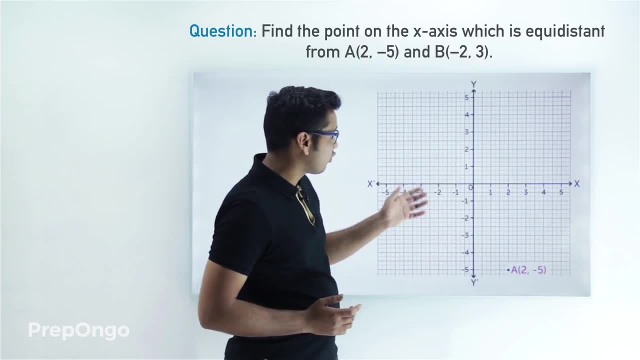 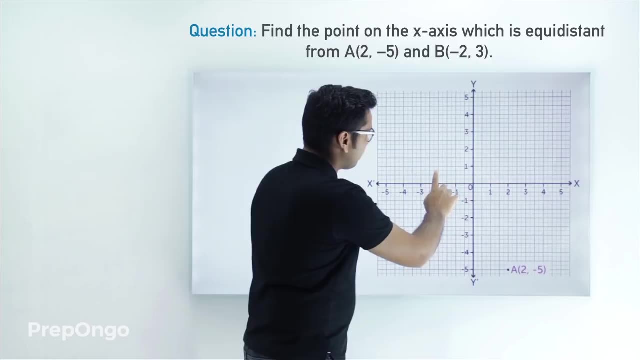 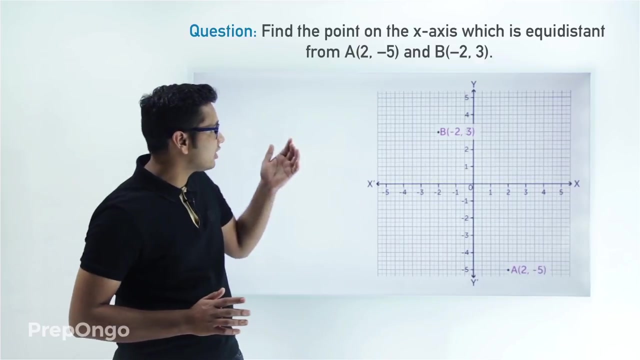 similarly we can plot B also. it is minus 2 comma 3. so we'll move 2 points on the negative x axis here and then we'll move up 3 points. so this will be minus 2 comma 3. now let's suppose that the point which is equidistant from these two 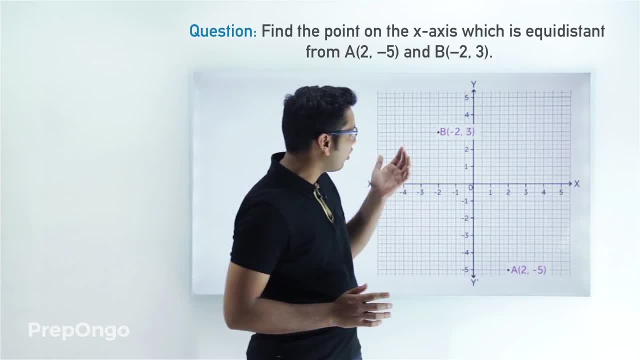 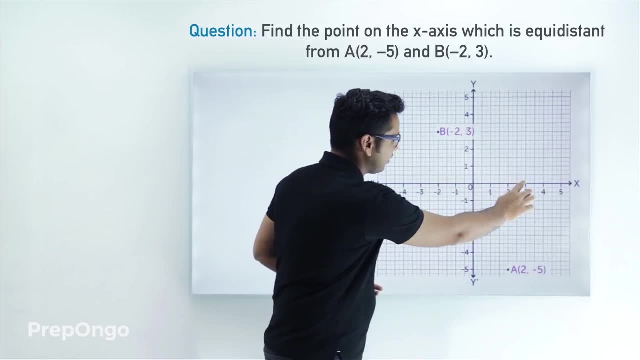 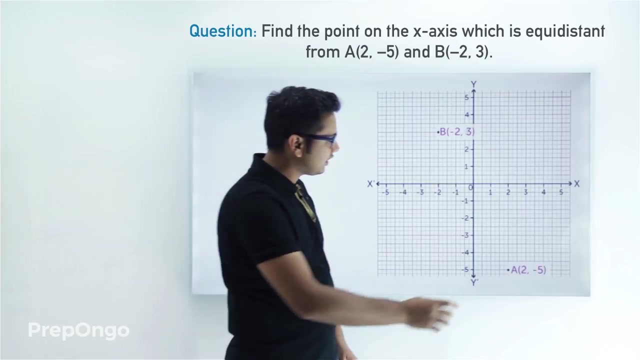 points is P, and since this is on x axis, you will find out that if a point is on x axis, it would be somewhere on this line, and if it is somewhere on this line, then the coordinates of Y will be 0. so let's say that the point is somewhere. 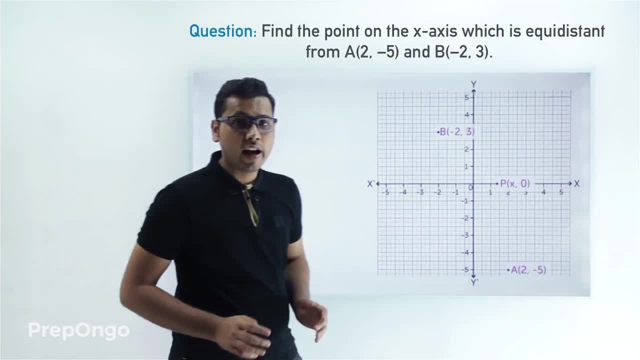 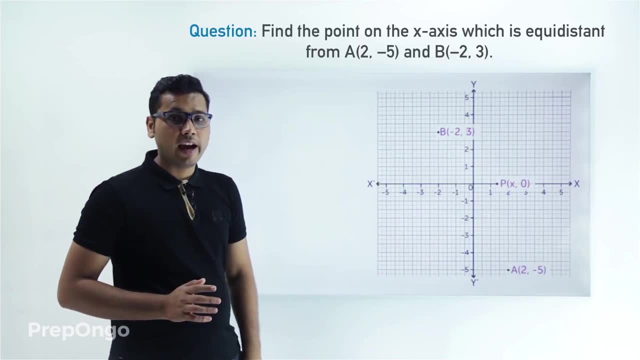 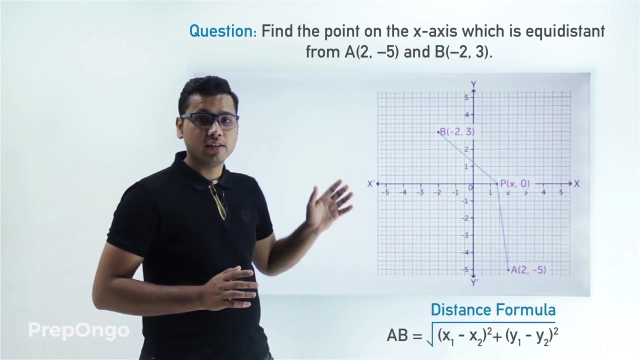 here, so its coordinate will become X comma 0. and now we can find out the distance PB and PA by using the distance formula and we will know that PA and PB will be equal. so let's apply the distance formula and get the distances PA and PB, and these distances will be equal. and then 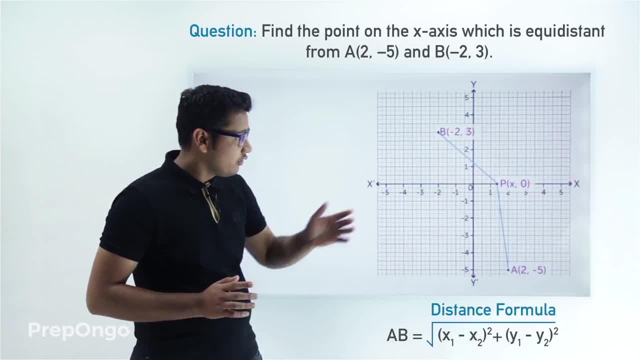 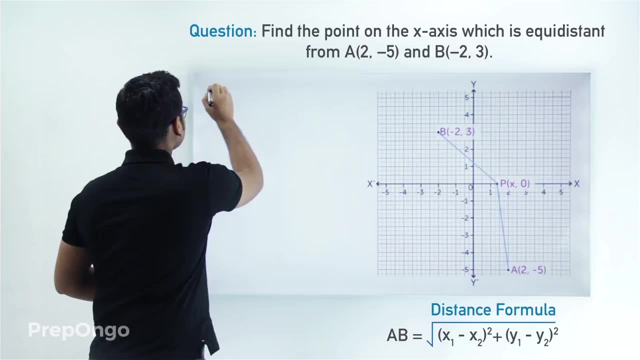 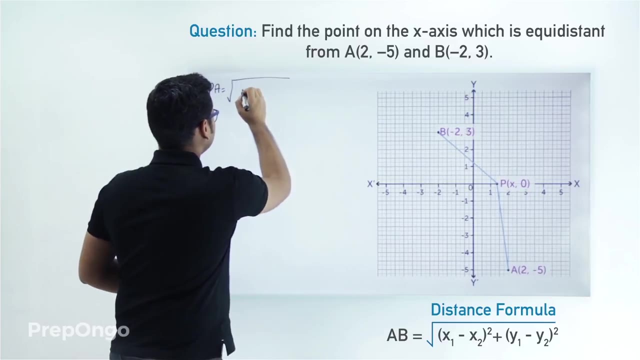 by equating them we can find out the coordinates of P point. so let's apply the distance formula here. so PA will be equals to under root of X 1 minus X 2, whole square. so X 1 is 2 minus X, whole square plus, and Y 2 is minus 5 minus 0, whole square. 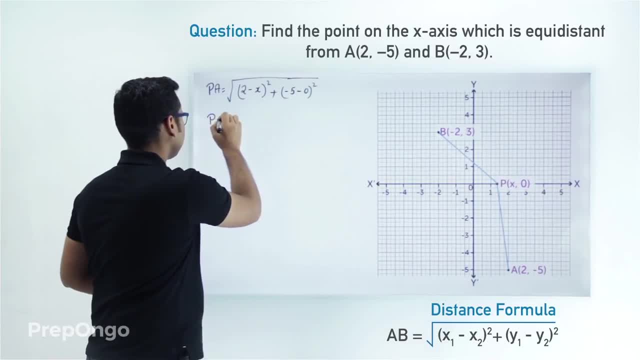 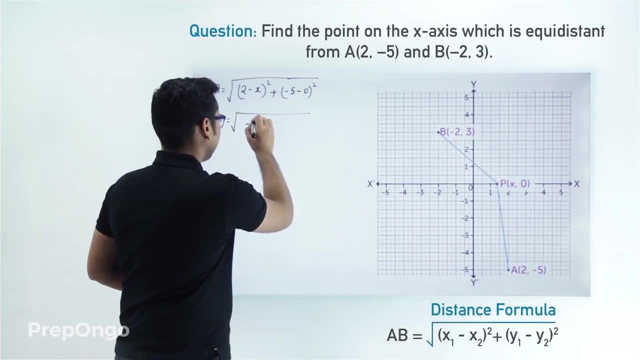 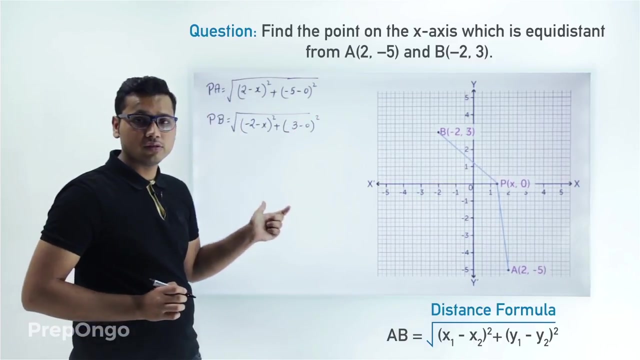 this will be PA. similarly, we can find out PB: PB will be equals to minus 2 minus X whole square plus and this will be 3 minus 0 whole square. and now we know we are given that these two are equidistant, so we can equate PA and PB. 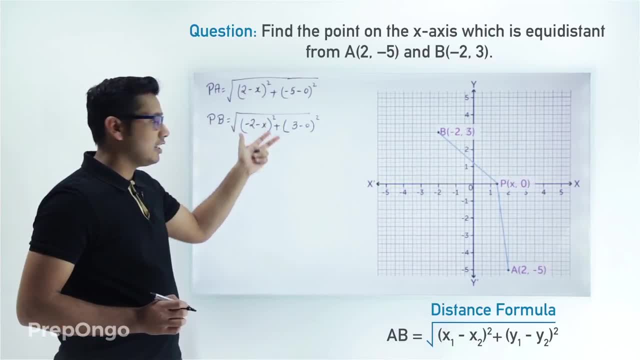 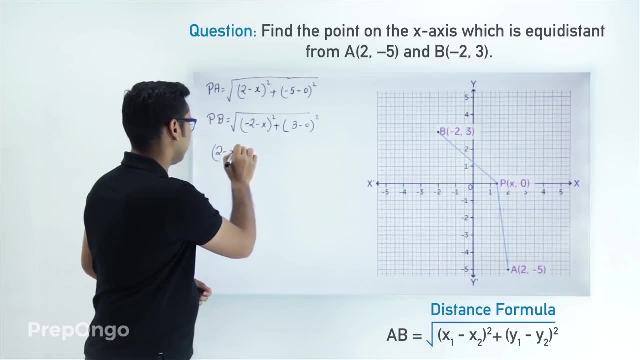 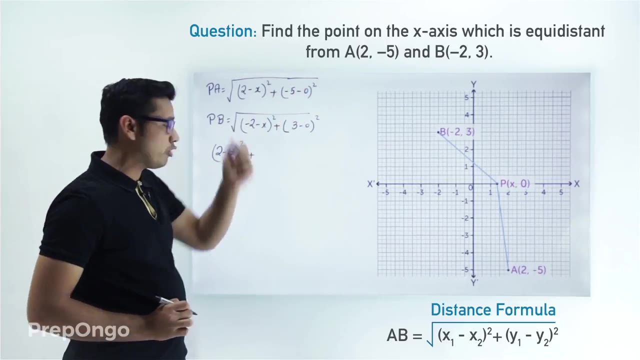 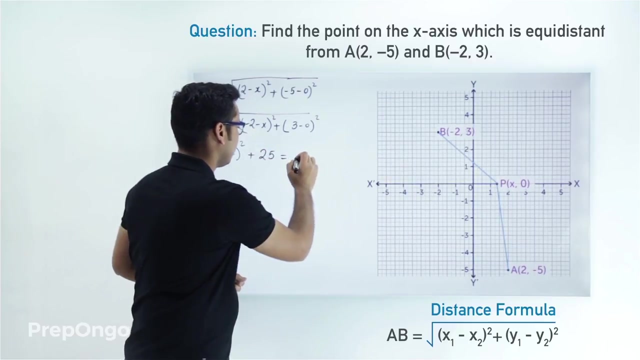 and these two quantities will be equal. so let's square and equate them so we can write down that 2 minus X whole square plus. if you look focus, this is minus 5 whole square. this will come out to be 25 and equals to this will be minus 2 minus X whole square plus. and let's square this, this: 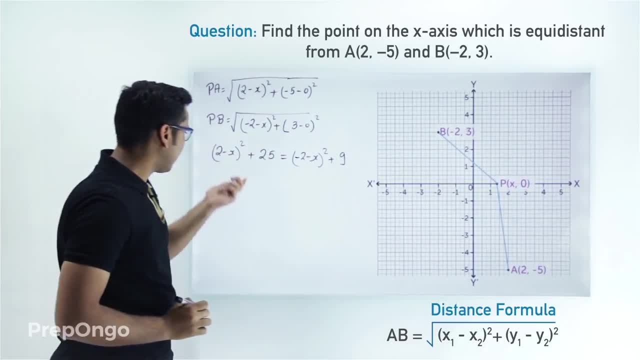 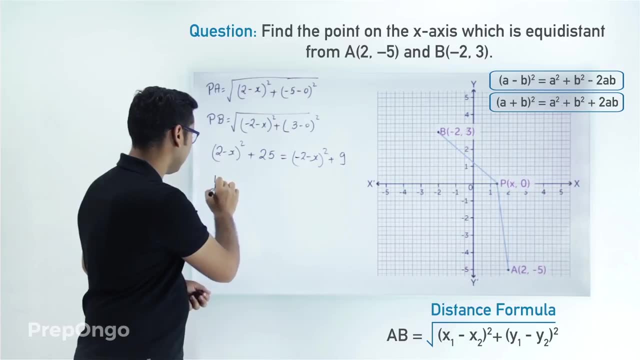 will come out to be 9. now just apply a minus B whole square here and a plus B whole square here, so this will be 4 plus X square, and minus 4x plus 25- equals to negative square- will go and this will become 2 plus X whole. 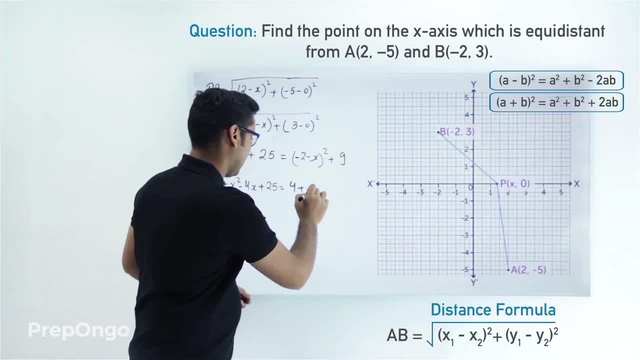 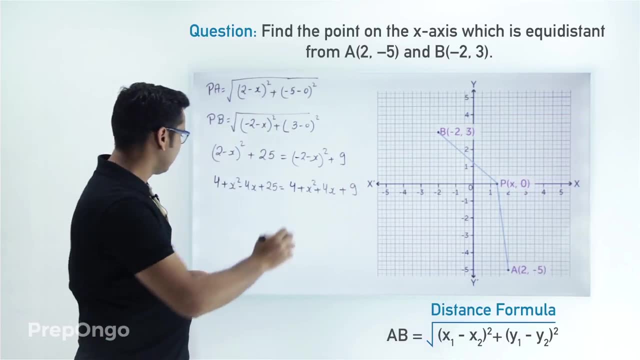 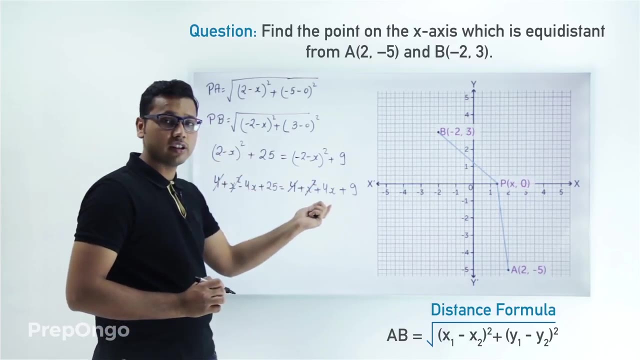 square. So let's solve this. This will be 4 plus x square, plus 4x plus 9.. Now, if we solve this, 4 will get cancelled. x square is also getting cancelled. Bring this: 4x on the right hand side and 9 on the left hand side, So this will be minus 9. 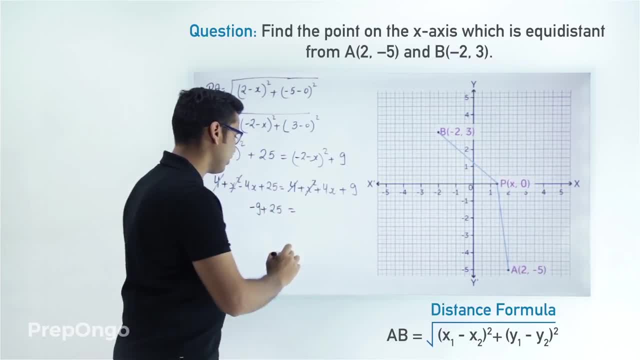 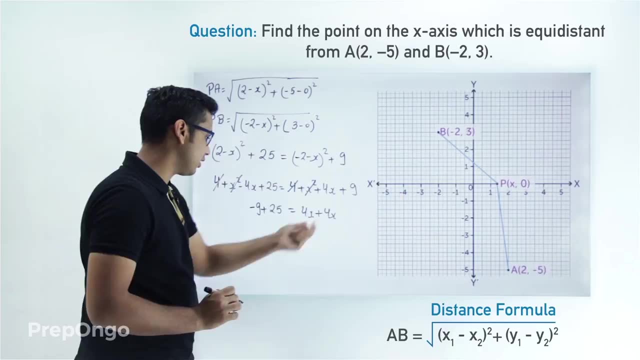 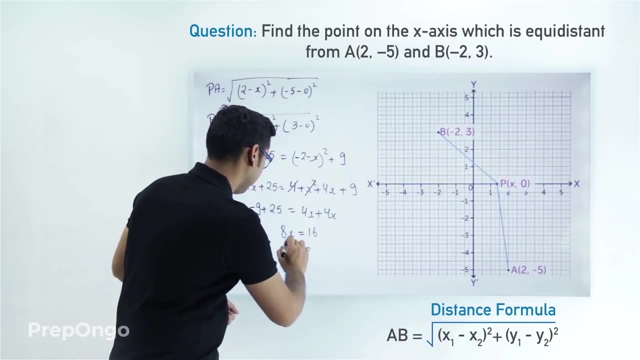 plus 25 is equals to 4x plus 4x. Just put this on the left hand side and take this on the right hand side, so this will be 8x equals to 16, or we can say x equals to 2, so we can say that the coordinates 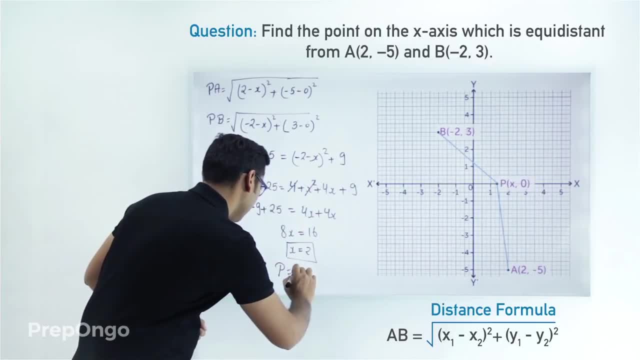 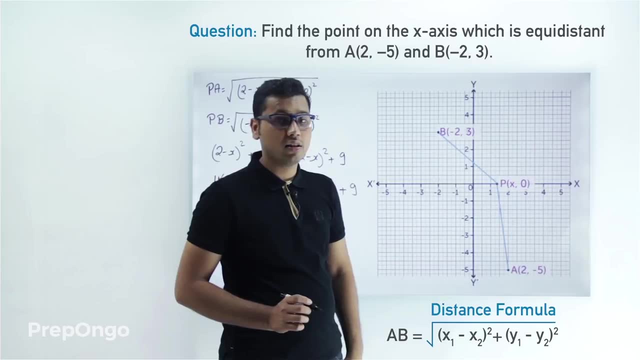 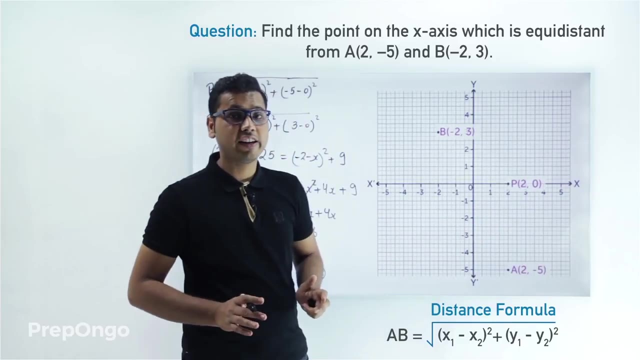 of P, point P will be equals to 2 comma 0. So this point P will not be here. rather, this will be here at this point, 2 comma 0.. So this is how we calculate the coordinates of a point which is equidistant from two. points.